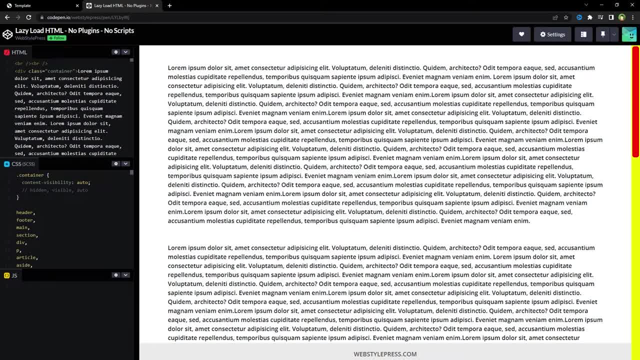 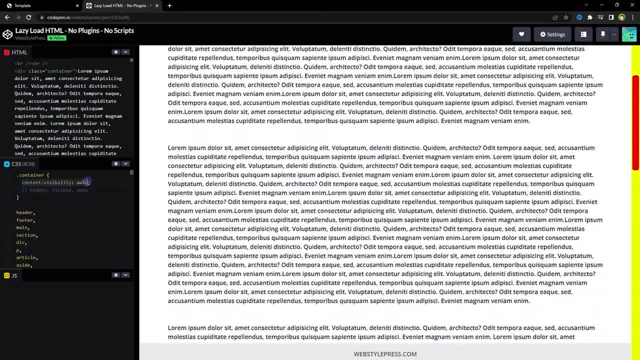 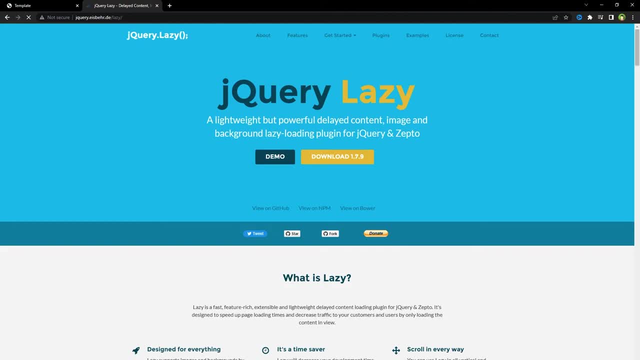 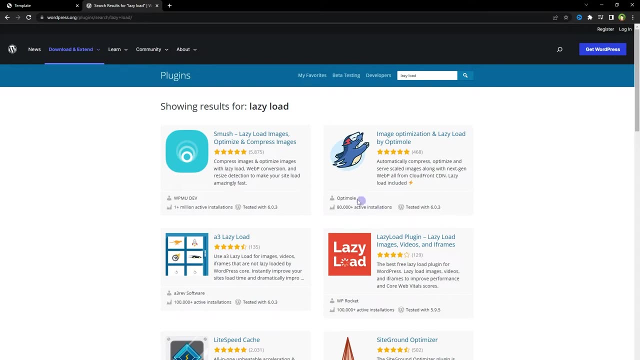 tutorials on this. For example, if we want to lazy load text or any element via only CSS, we have Content Visibility Auto in CSS. We have jQuery plugins to implement lazy loading For WordPress. we have WordPress plugins for lazy loading, For example, Smush Image Optimization Lazy Load. 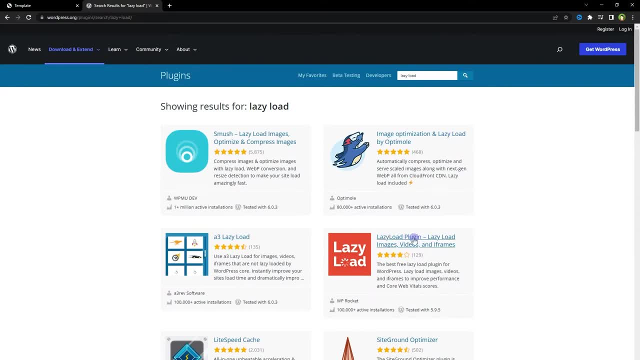 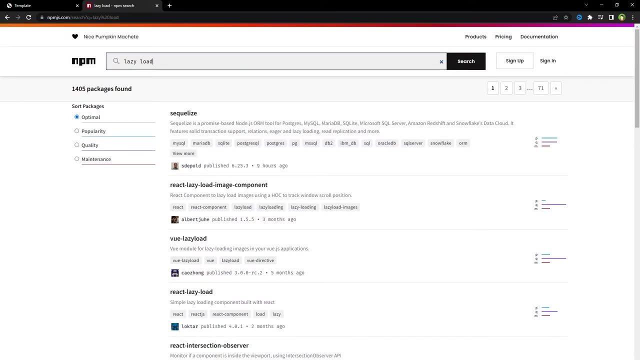 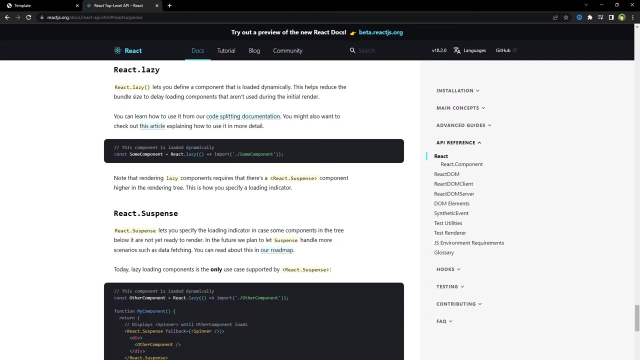 A3: Lazy Load. Lazy Load Plugin and more. Many cache plugins also provide lazy loading For JavaScript-based applications. you can also use Lazy Load For JavaScript-based applications. we have Lazy Load packages for ReactJS, VueJS and more For ReactJS specifically. 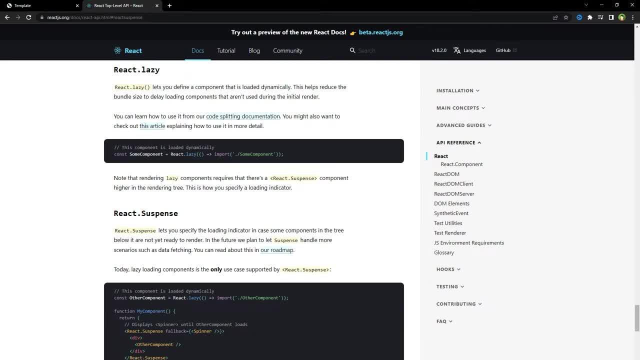 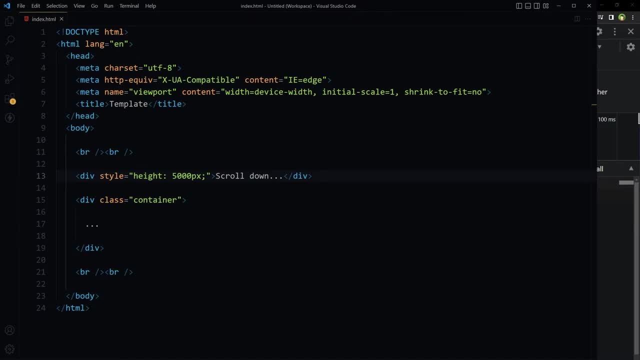 we have ReactLazy and ReactSuspense components for lazy loading, So there are many ways to implement lazy loading in CSS, in JavaScript, in ReactJS, in jQuery, in WordPress and more, But there is a way that can be used to lazy load elements without CSS, jQuery or JavaScript. 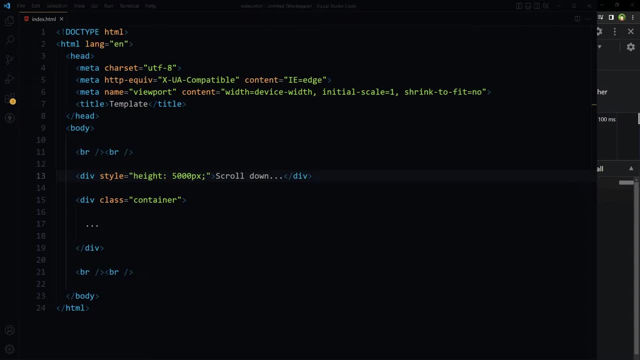 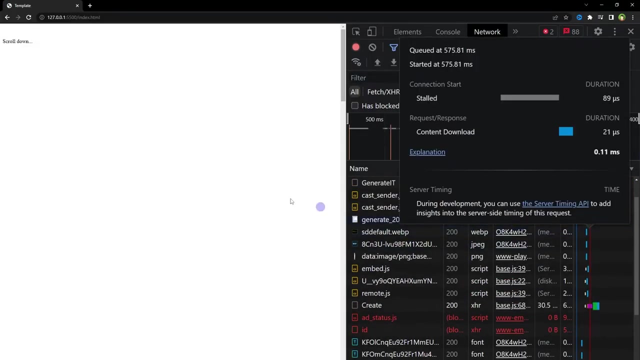 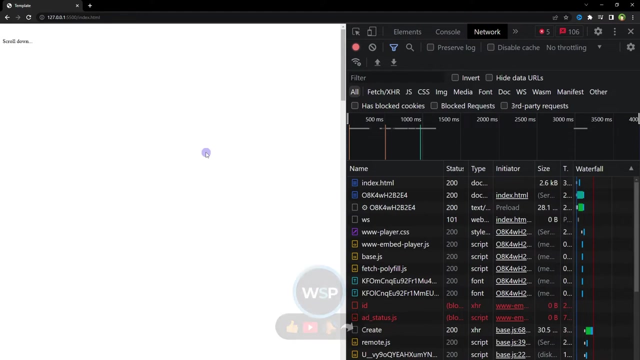 It is native lazy loading. For example, we have this HTML and the output is here. We have this iframe. It's a video. If I save this, it is already loaded in DOM. This is a video from YouTube Reload page. Video is loaded. 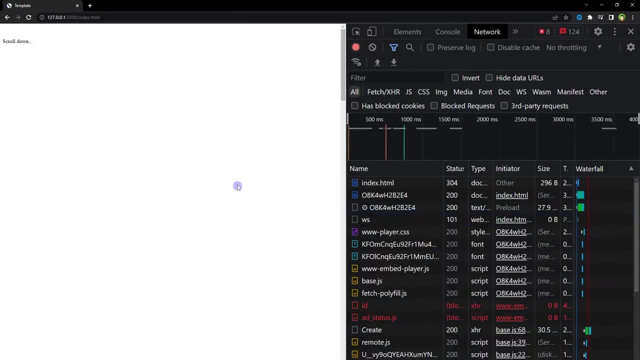 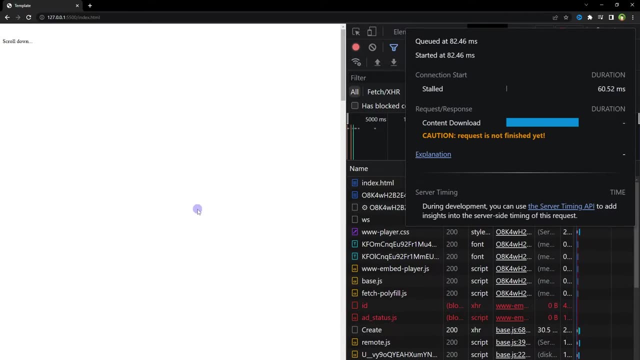 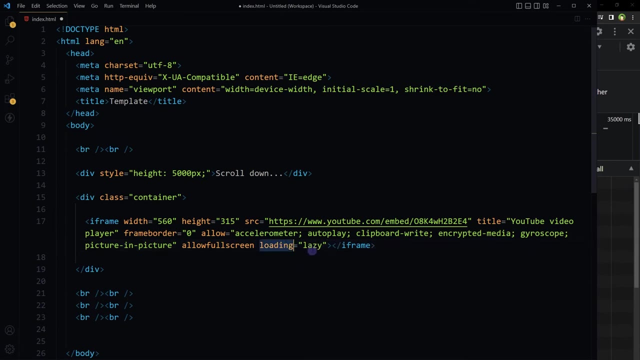 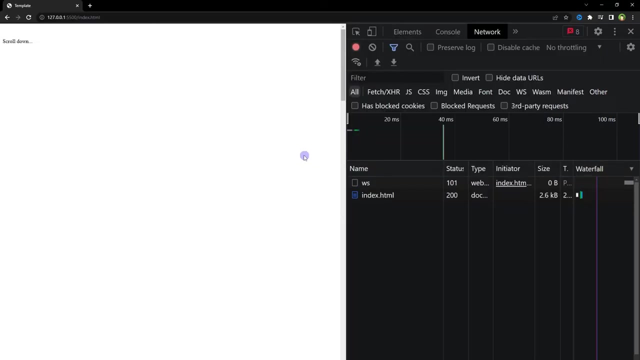 Reload page. Video is being loaded. To see these we'll have to inspect element and go to Network tab. So if we refresh the page, iframe loads in DOM. But if we apply loading attribute with lazy value and save it, then it is not loaded. 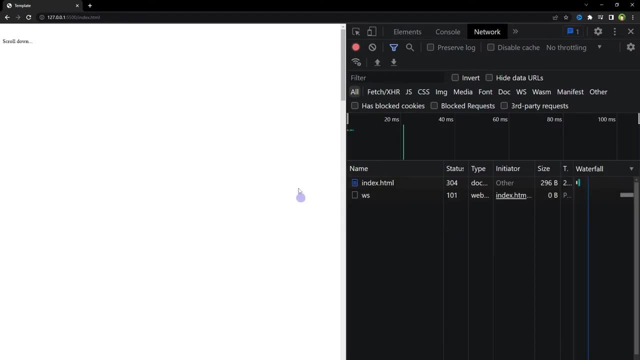 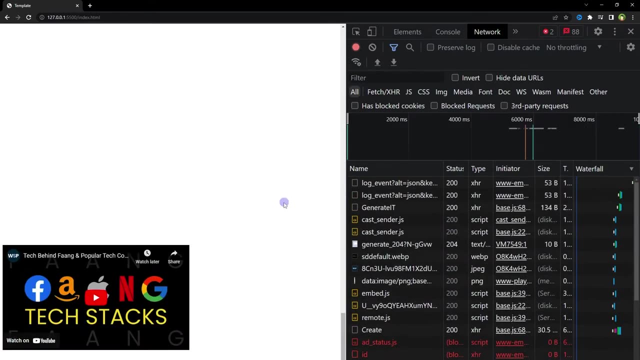 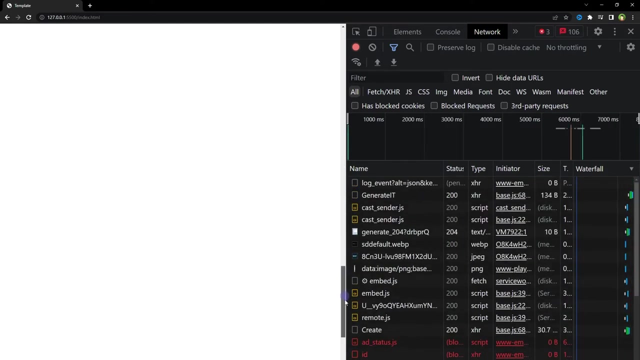 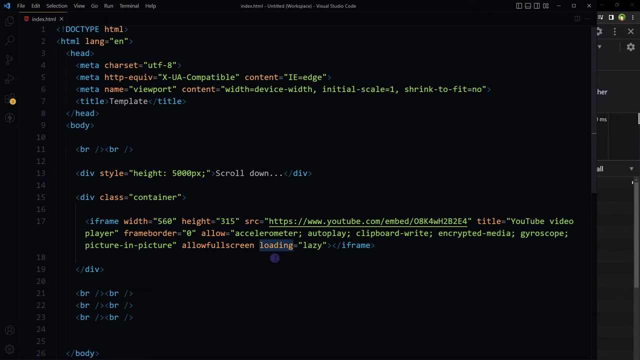 Reload, Reload And a video is not being loaded, Plus writing the мен Examples, Unless we scroll near video Or near this iframe. Let's see this again. Reload the page, Scroll to the iframe And it is loaded. Reloading attribute can be used to instruct the browser to defer loading of images and 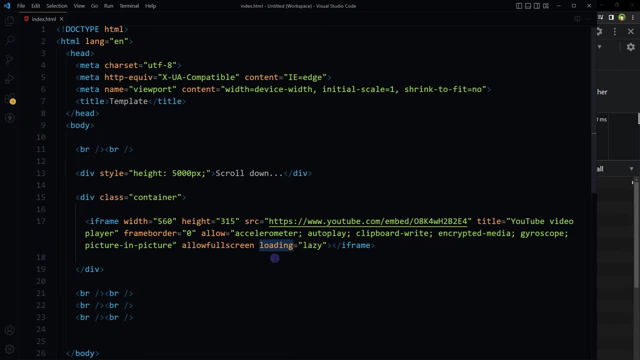 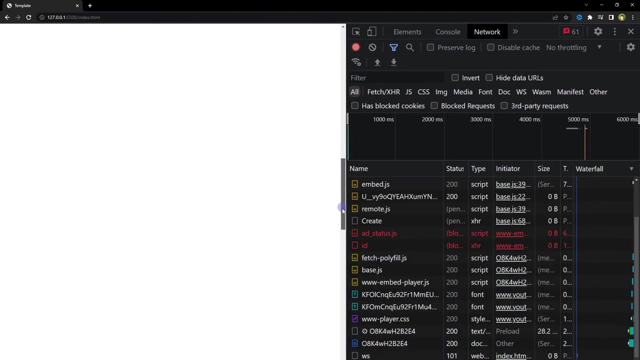 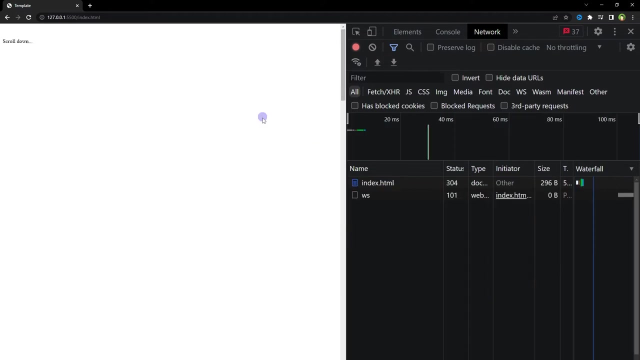 iframes that are offscreen until the user scrolls near them And for image, We can add the image tohim And we can discard the images from this iframes. We can apply the same attribute: See. image is not loaded. 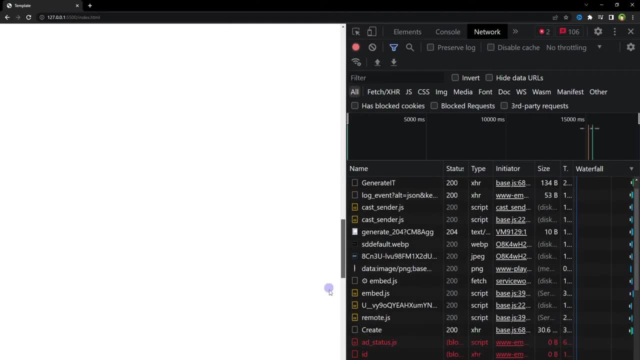 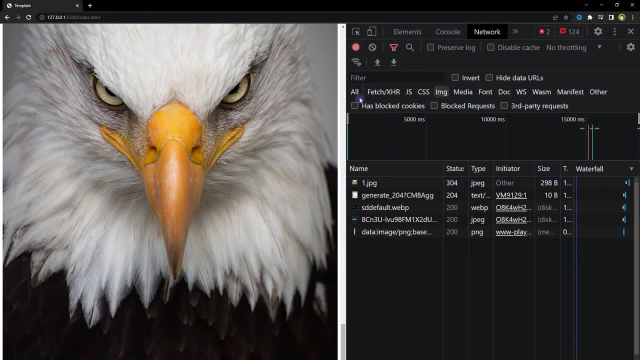 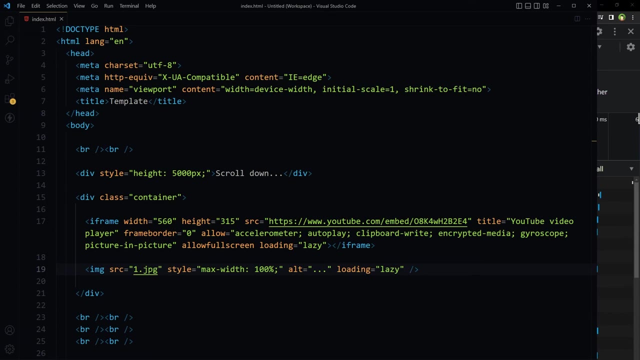 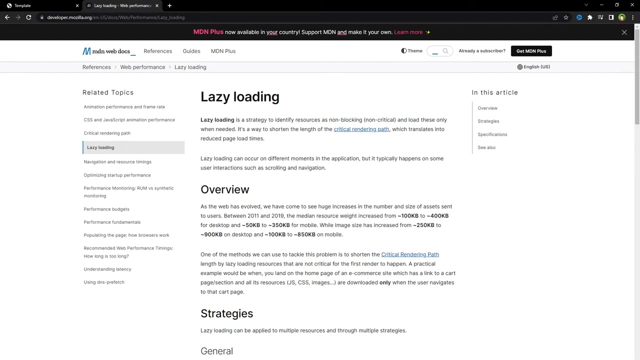 Iframe is not loaded. If we scroll down, then the image is loaded. The load event fires when the eagerly loaded content has been loaded. So lazy loading images and iframe is possible by using loading attribute with lazy property in HTML elements. For more on this, go to MDN website and look for lazy loading. 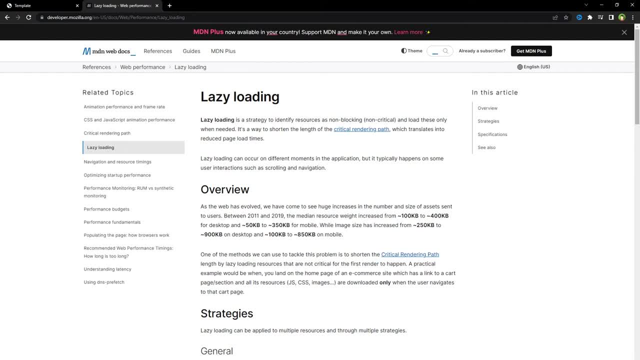 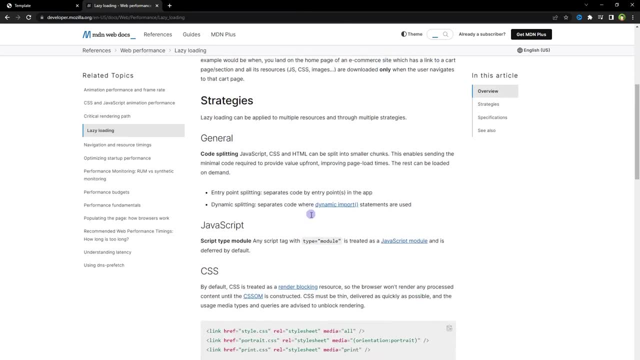 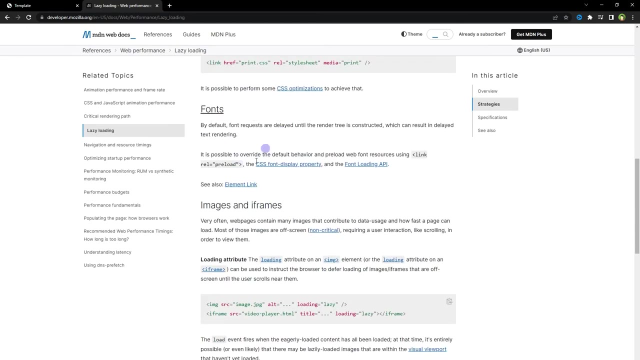 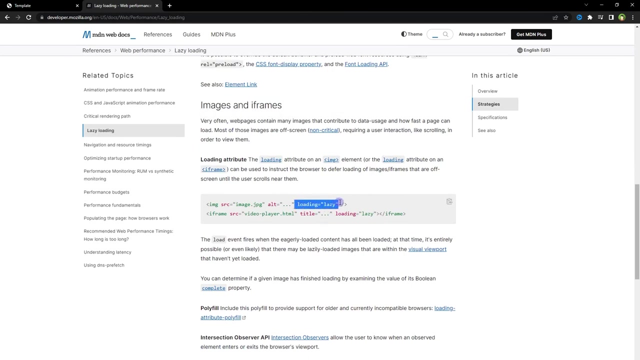 Here we have detail on lazy loading. Lazy loading strategies for CSS for JavaScript: fonts, images and iframe. Strategies for JavaScript by using type module For fonts: rel preload For images and iframes loading lazy- Native lazy loading is available for images and iframes. 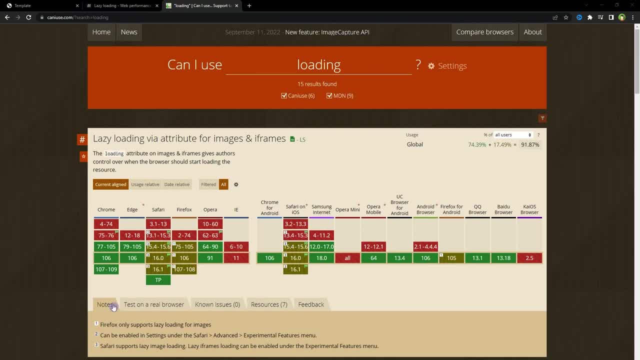 Support for loading lazy is available. It's available for Chrome for Edge. for Safari: It's available for Safari technology preview. Firefox only supports lazy loading for images, not for iframe. Opera supports it. Chrome for Android supports it, So support for loading lazy is being added gradually. 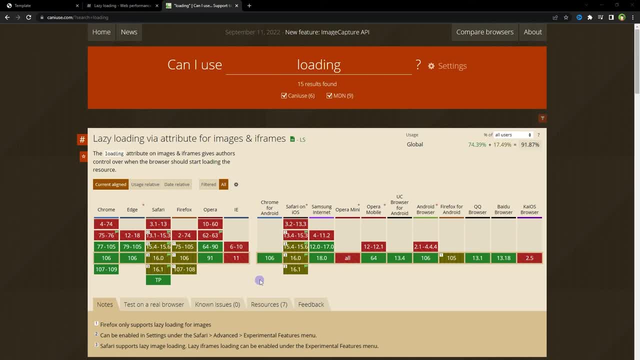 Okay, I hope it helped. Like, share, subscribe and I will see you in the next video. Thanks for watching.